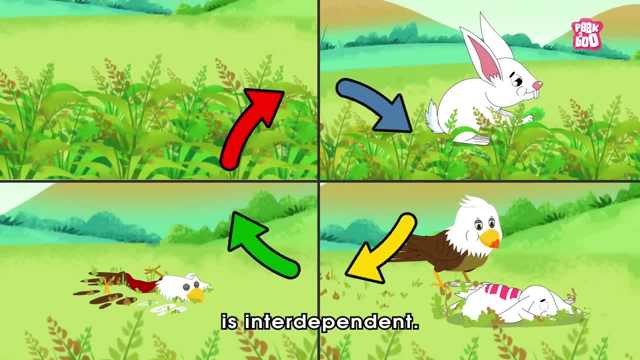 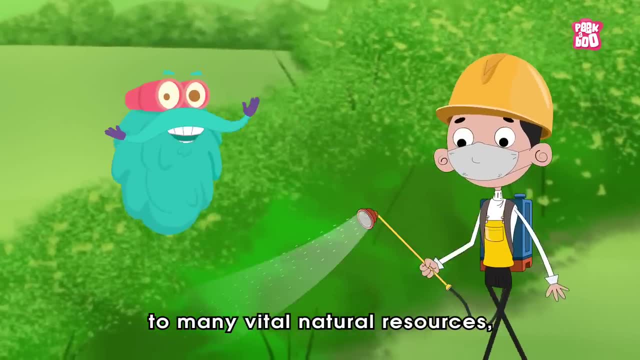 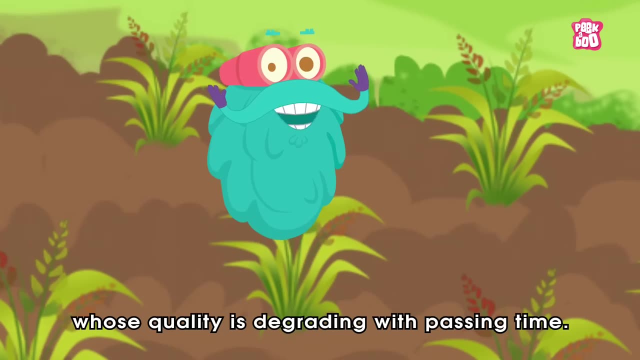 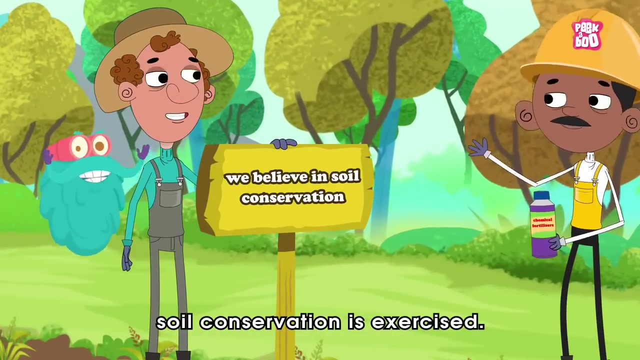 and everything around us is interdependent, but this dependency sometimes proves harmful to many vital natural resources, and one of these resources is soil, whose quality is degrading with passing time. So to stop this degradation of soil, soil conservation is exercised. and what is that? 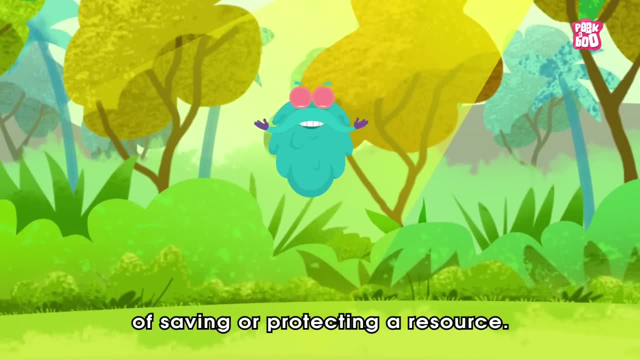 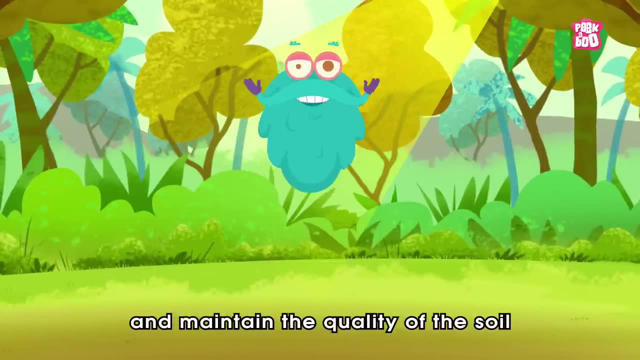 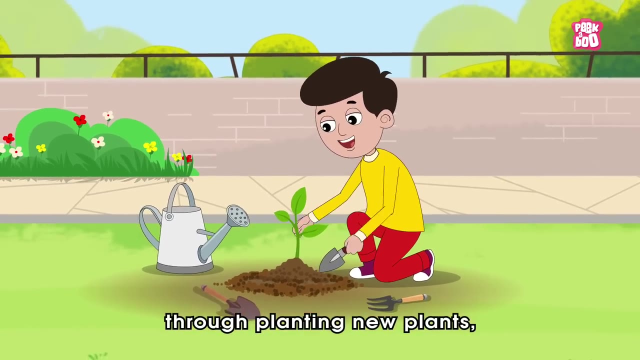 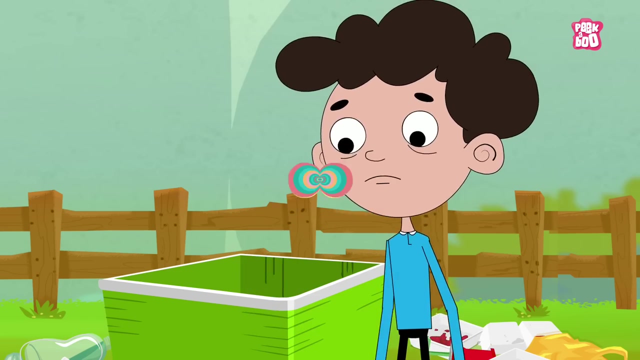 Well, conservation is the act of saving or protecting a resource, and soil conservation is a practice that helps to retain and maintain the quality of the soil by preventing soil erosion through planting new plants, taking care of plants or keeping soil from being contaminated. But the crucial question is: why is it required? 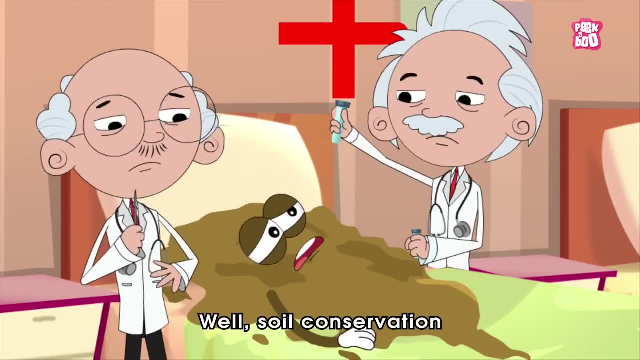 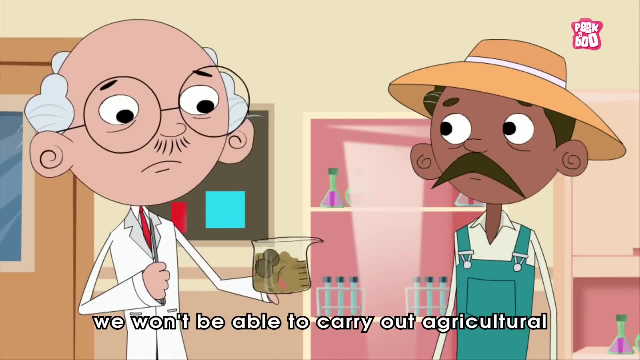 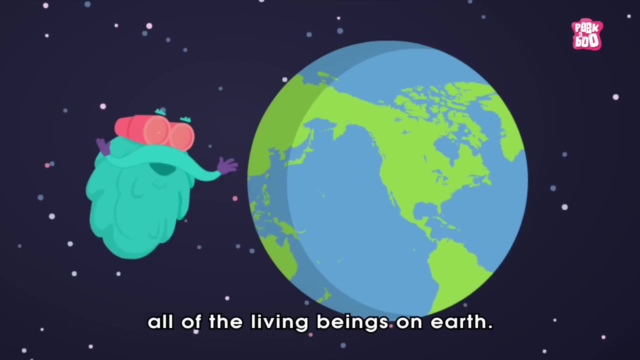 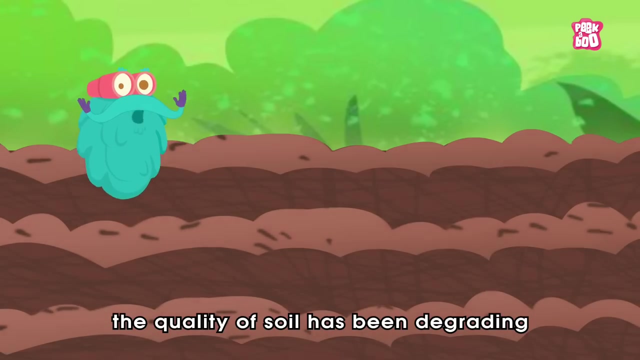 In the first place. well, soil conservation is necessary because if we run out of healthy soil, we won't be able to carry out agricultural and planting activities that are necessary to feed all of the living beings on earth. And unfortunately, in recent times, the quality of soil has been 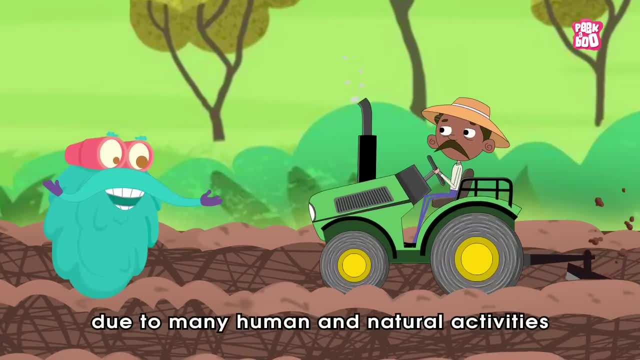 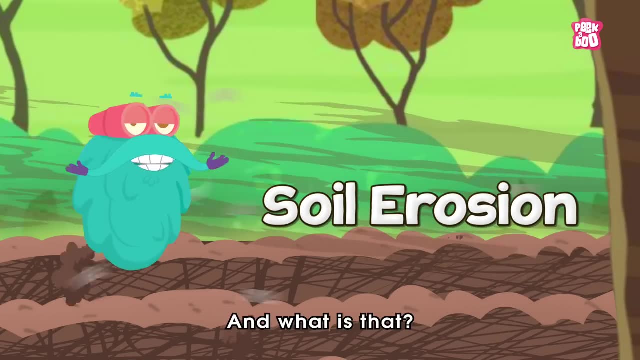 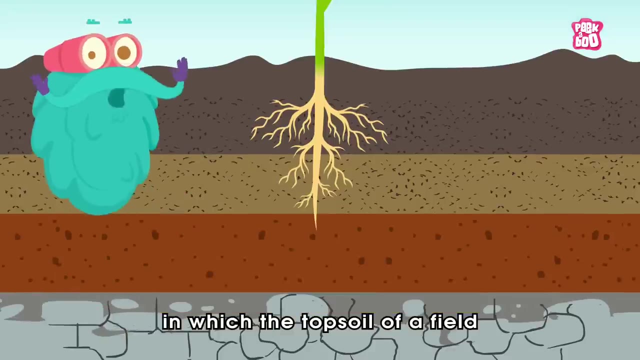 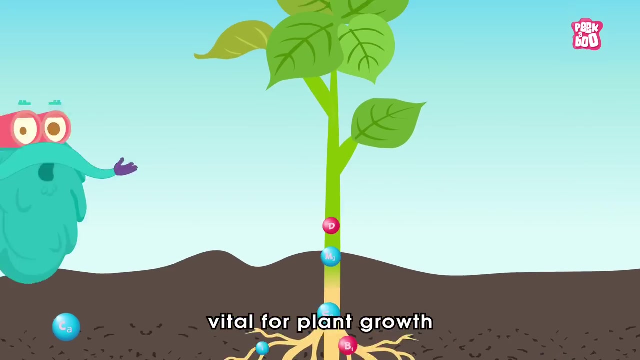 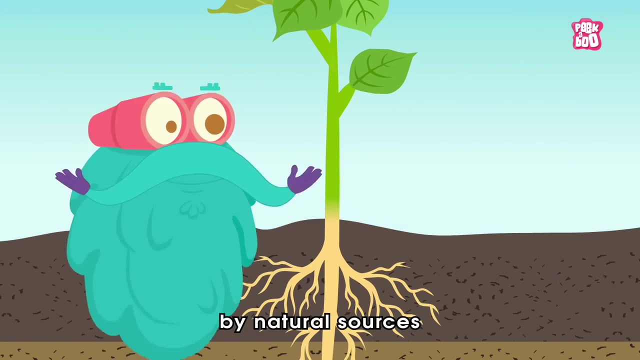 degrading at an alarming rate due to many humans. Soil conservation is a process in which the topsoil of a field, containing the highest number of nutrients, microorganisms and minerals vital for plant growth, is washed away from one place to another by natural sources such as wind and water. 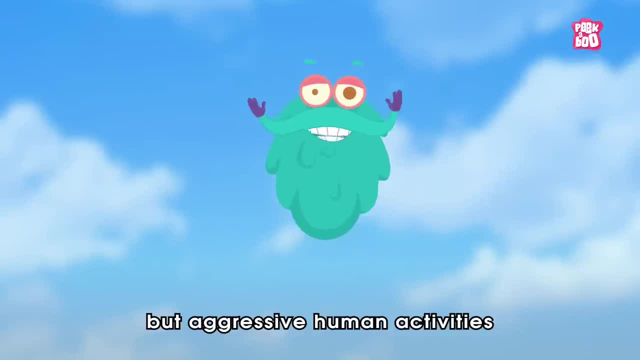 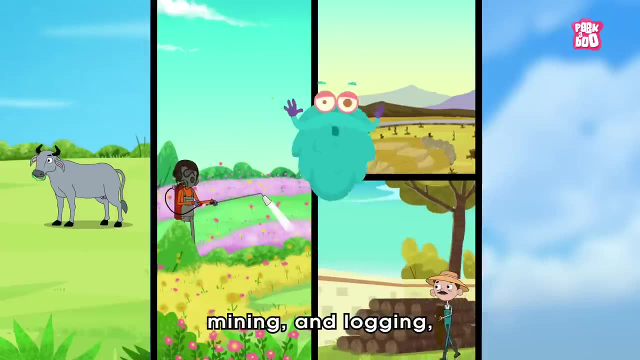 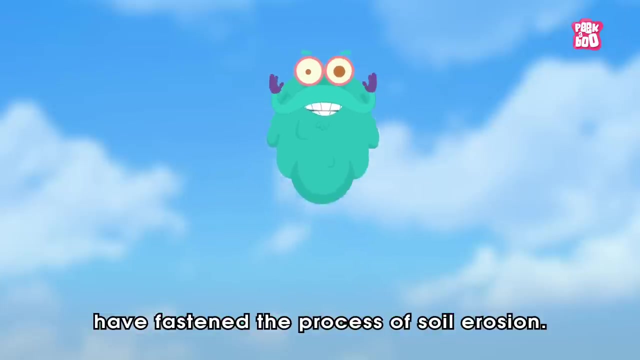 Not only that, but aggressive human activities such as overgrazing of cattle, overuse of pesticides, mining and logging, construction of roads and buildings have fastened the process of soil erosion, So the need for soil conservation has increased more than ever before.